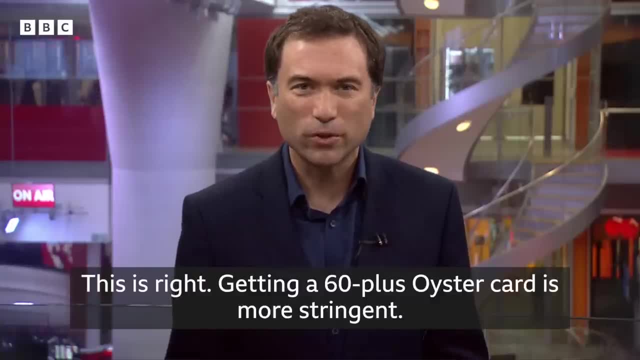 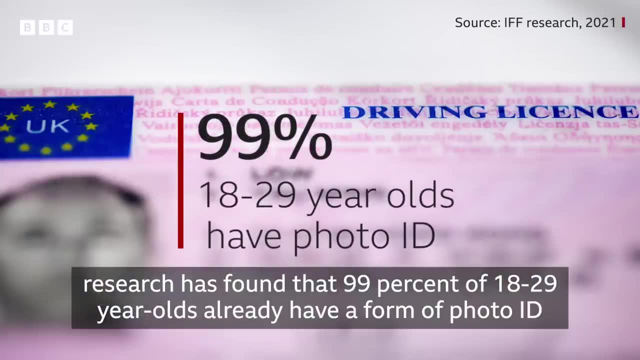 This is right. Getting a 60-plus Oyster card is more stringent And, while younger people can't use their Oysters to vote, government commission research has found that 99% of 18-29-year-olds already have a form of photo ID that can be used. 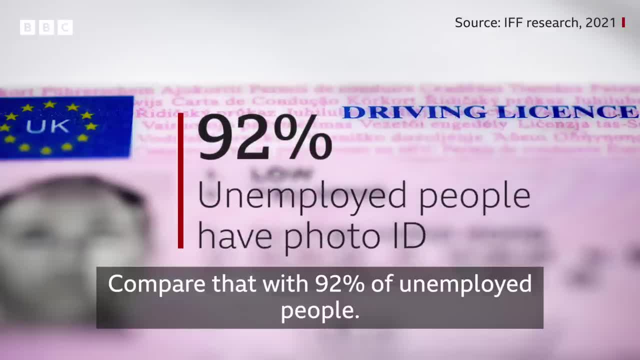 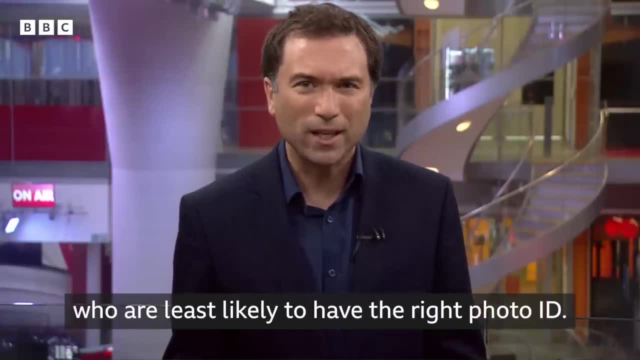 Compare that with 92%- 92% of unemployed people. The data suggests it's disadvantaged groups, not young people, who are least likely to have the right photo ID. And if we look at this more broadly, BBC analysis of Electoral Commission data calculates that 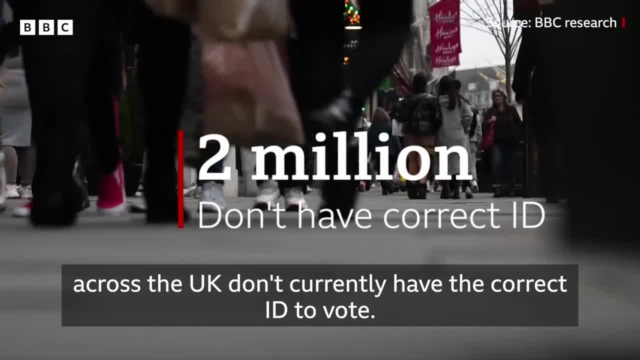 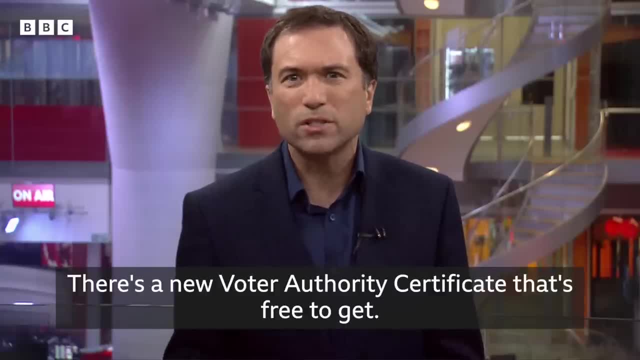 almost 2 million people across the UK don't currently have the correct ID to vote. Now the government says it's trying to address that. There's a new voter authority certificate that's free to get And so far There's a new voter authority certificate that's free to get. 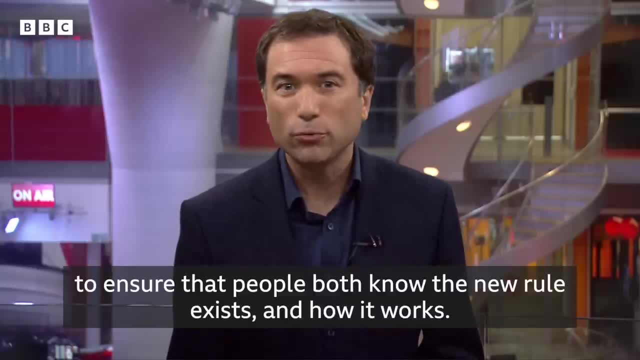 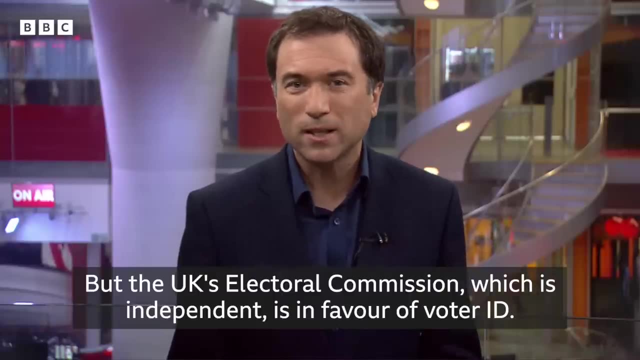 Evidently, there remains work to do to ensure that people both know the new rule exists and how it works, But the UK's Electoral Commission, which is independent, is in favour of voter ID. In a 2014 report, it said: 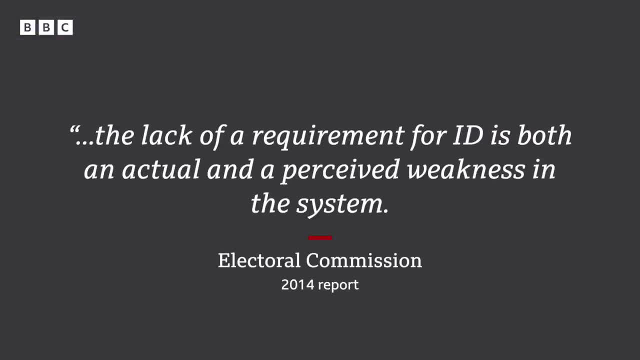 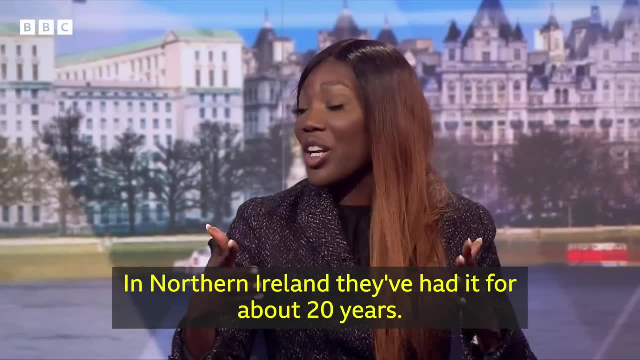 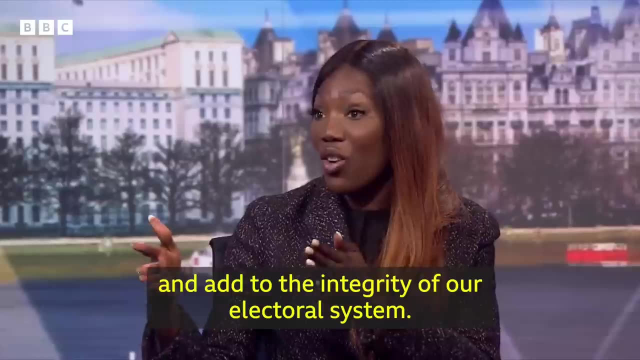 And this former Tory adviser is convinced We use ID when we go to collect a parcel In Northern Ireland. they've had it for about 20 years. Like there are very reasonable things that you could see in the long term would benefit and add to the integrity of our electoral system. 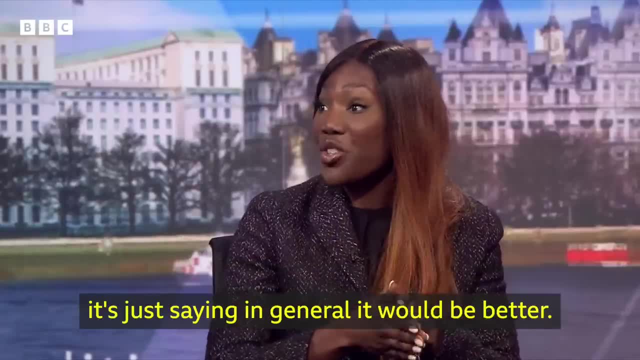 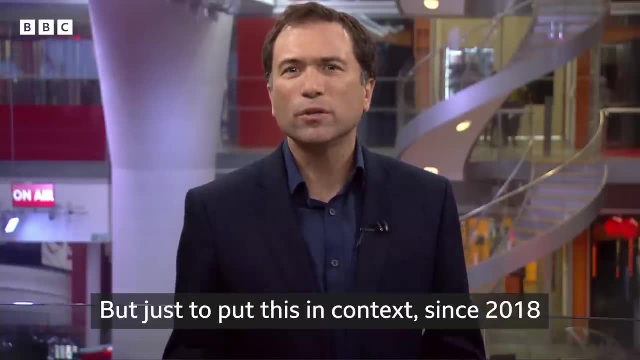 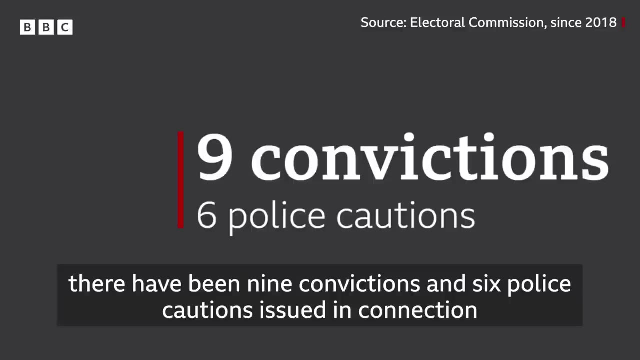 That's not about saying the system is currently rife with fraud. It's just saying, in general, it would be better. The government, too, says voter ID is protection against potential election fraud. But just to put this in context, since 2018, there have been nine convictions and six police cautions issued in connection with cases of electoral fraud. 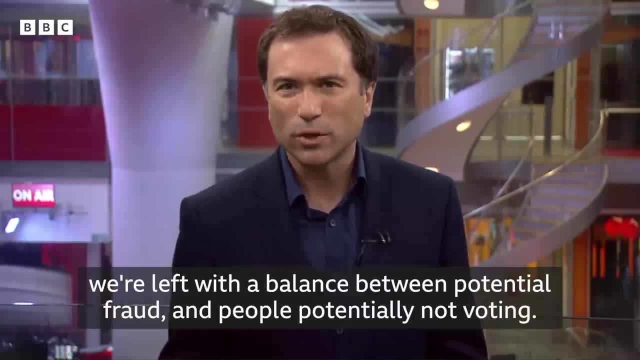 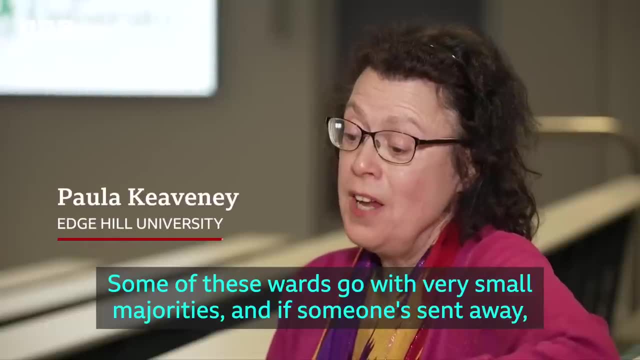 That's a tiny fraction of the electorate, And so we're left with a balance between potential fraud and people potentially not voting. Some of these wards go with very small majorities, And if someone's sent away and they think I'm not coming back with the ID, I can't be bothered. 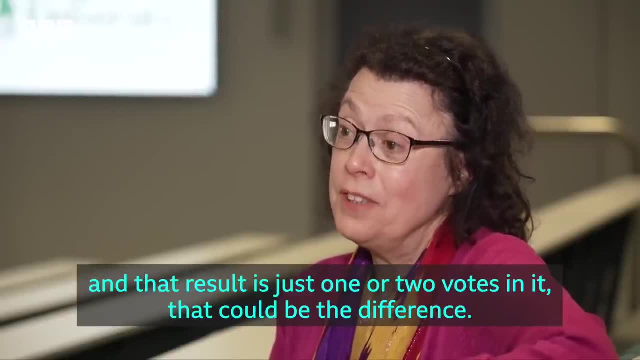 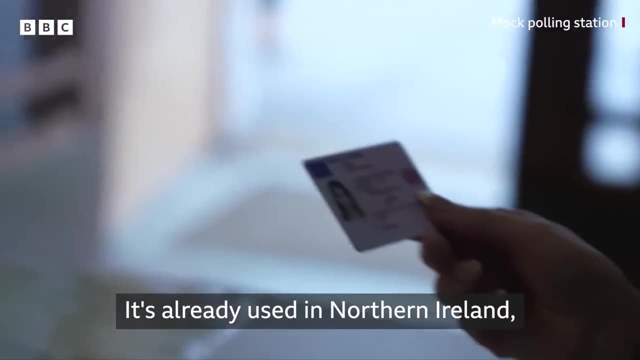 and that result is just one or two votes in it. that could be the difference. It could be the difference, But it's worth noting that voter ID is not unusual. It's already used in Northern Ireland, as it is in France, Italy, Canada and other Western countries too.